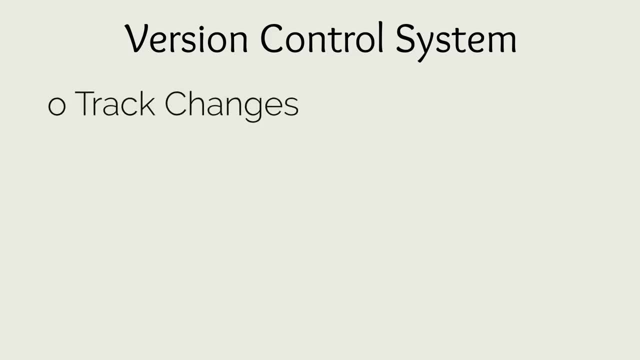 tracking changes to your code over time, painless. Git tracks every change that has ever been made to the code you tell it to manage and lets you easily switch between versions of your code or even undo changes. Git also makes it easy for teams of people to work on the same project and 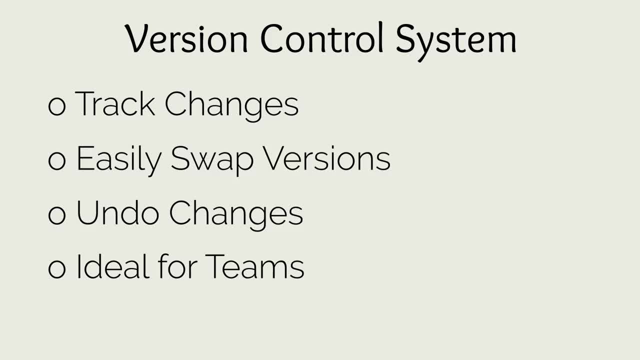 even the same file, since each team member has their own version of the code saved locally on their computer. Git also saves the full version history on each team member's computer, which is what makes it a truly distributed version control system. This is all great, but teams need a place. 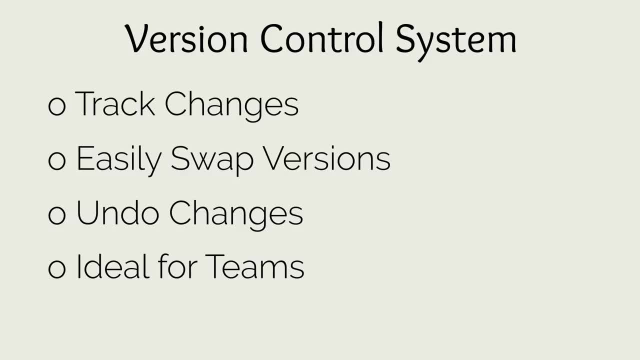 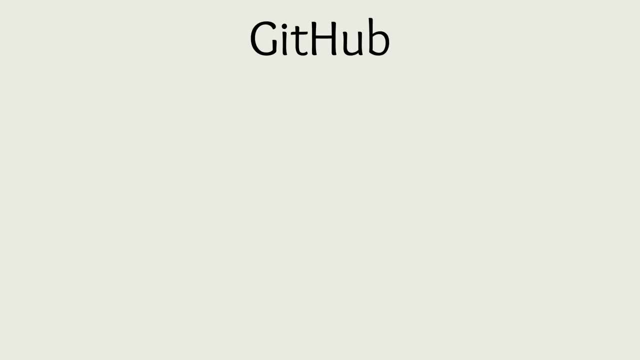 to store their code remotely so that all the team members have a central place to save their changes to and pull down other team members' changes. This is where GitHub comes in. Many people get confused when they first learn about Git and GitHub, thinking that they are the same thing. 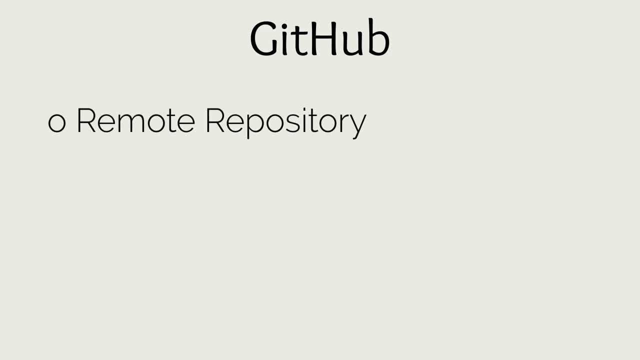 However, GitHub is just a website where developers can store their projects for other developers to access. Git, on the other hand, as we talked about, is just a version control system for tracking and managing changes to code. Now that we have a basic understanding of what Git is, 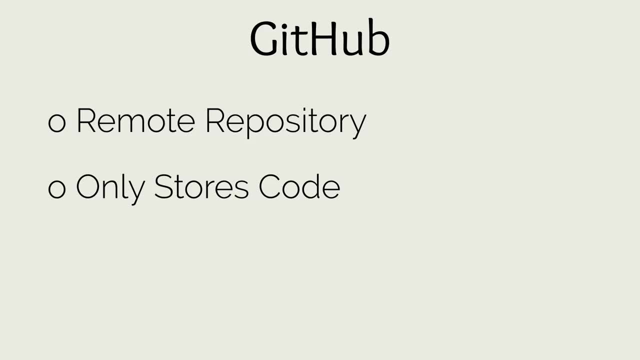 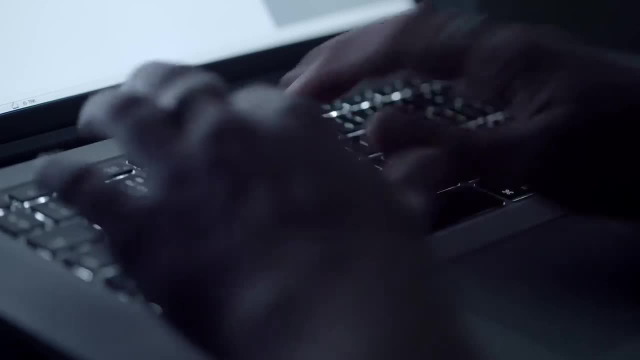 let's jump into why Git is so important. Git is a version control system that allows you to use Git on all of your projects. Imagine the scenario where you are working on a multi-part YouTube tutorial to learn the basics of HTML, such as my Introduction to HTML course- and you 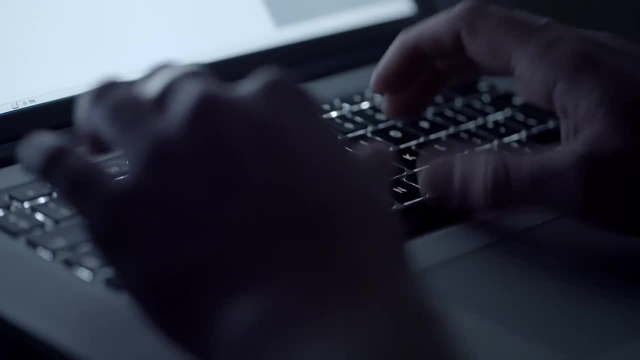 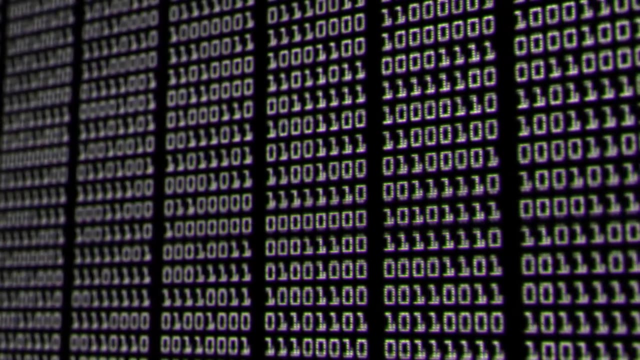 just finished writing all of the code for one of the middle videos in the series, only to find out that something you did broke everything. Without Git, you would have to resort to trying to remember what you changed since the previous video and then search through each of those files to determine. 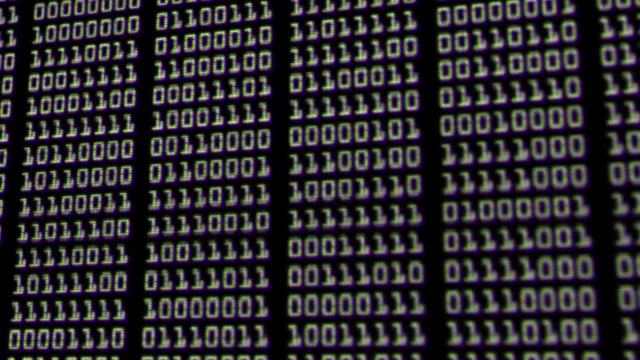 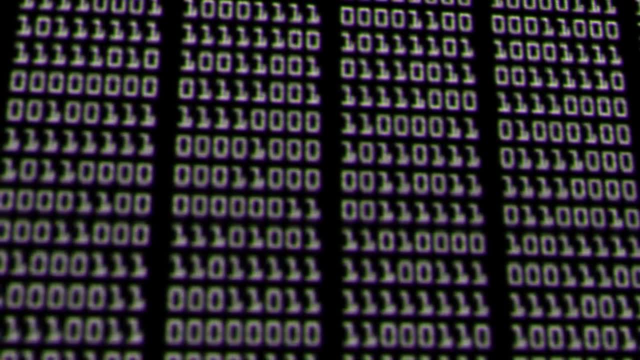 what exactly is wrong. If you're lucky, you'll remember all the changes that you made, but most likely you'll have to remember what you changed since the previous video and then search through all of the files of the project looking for a single mistake. With Git, though, this is a trivial. 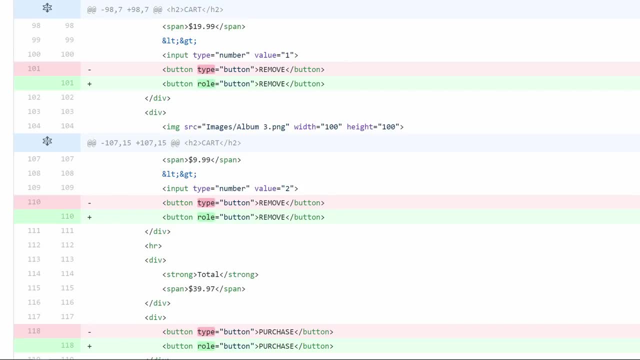 problem to solve, since Git tracks all the changes that you make. You would simply have to tell Git to show you all of the changes that have occurred since the previous video's code, and Git will not only show you what files have changed, but will also show you the exact changes that have occurred. 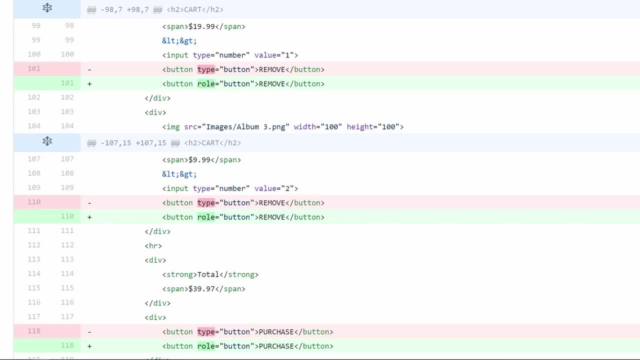 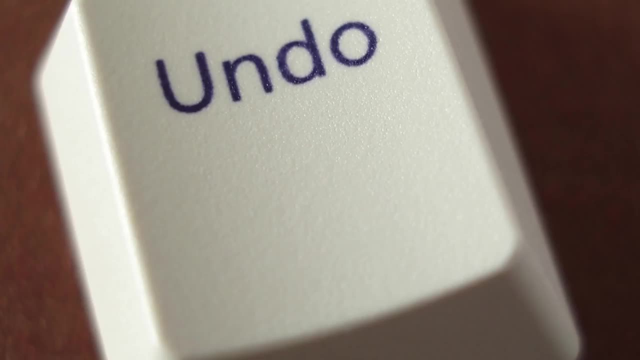 in each file. This makes finding what went wrong more enjoyable and quicker. Git also allows you to change back to previous versions of your code with a single command. This is extremely useful for any project, since if you deploy your changes to the world and realize later that something major is, 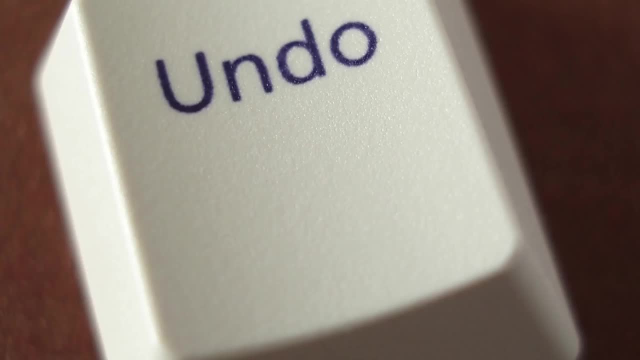 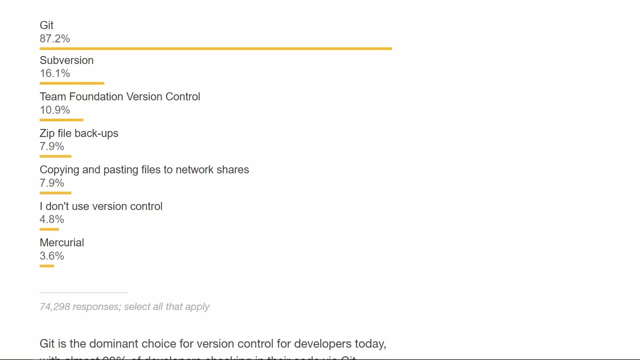 broken, you can simply tell Git to change back to the previous non-broken version of your code. Without Git, this is an impossible task, since nobody will perfectly remember all the things that need to be reverted to get back to the previous version. Lastly, Git is used by nearly all developers with Stack Overflow reporting that nearly 90% of 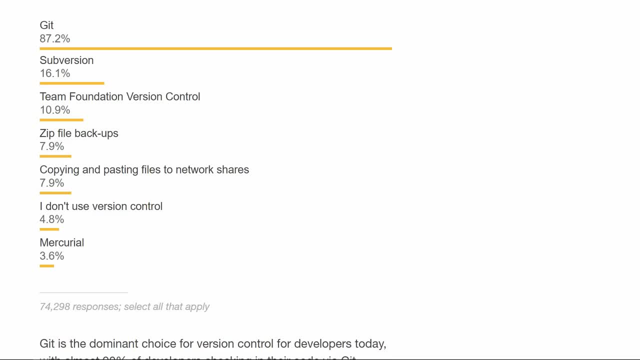 their 75,000 developers they surveyed used Git as their version control system. This means for anyone looking to get a job in programming, they will need to know Git. Lastly, you need to ensure that Git is installed on your system and configured with your GitHub account, If you do not already. 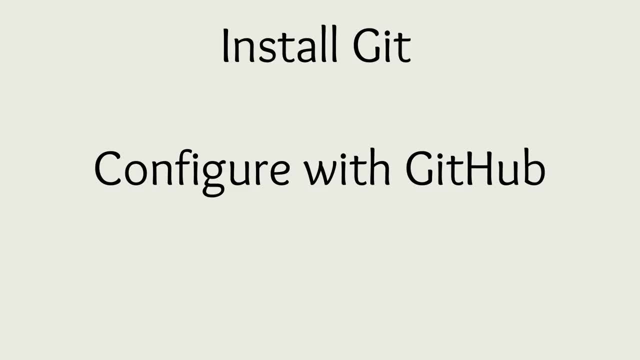 have Git installed or do not have Git linked with GitHub, then check out my video on the introduction to web development, where I cover installing and setting up Git with GitHub. This will be linked in the description below. Now that you have Git properly installed and set up with GitHub, we can 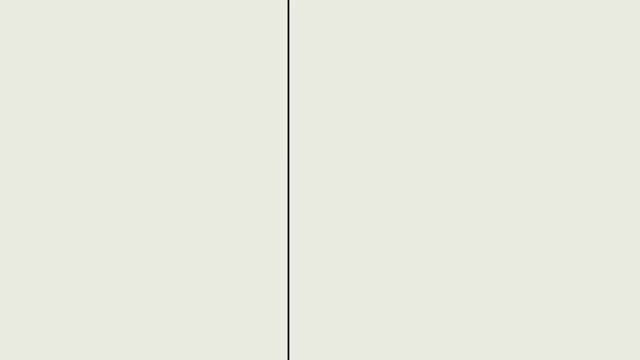 begin talking about how to use Git, The first thing you need to do is initialize Git in your existing project from a website such as GitHub. In order to initialize Git in a project that already exists on your computer, simply run the git init command in the terminal from the folder that contains. 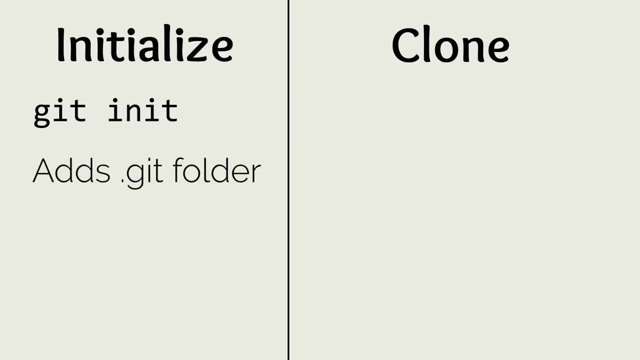 all of your project files. This will add a git folder to your project that Git will use to track all the changes you make to your project. Git also uses the word repository, or repo for short, to describe the entire project being managed by Git. 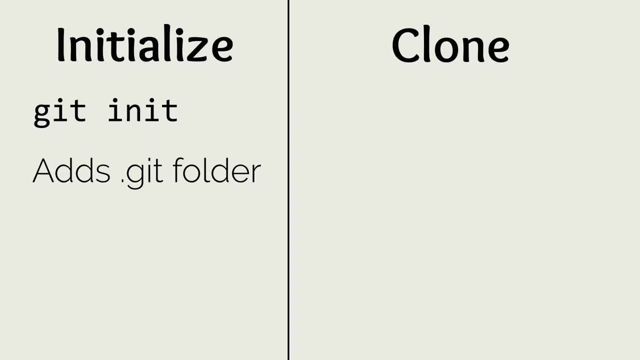 The second option of cloning a repository can be done by going to GitHub and either creating a new repository to clone or finding an existing repository and copying the link to clone the project. If you set up Git in GitHub using the method from my video, make sure to copy the ssh. 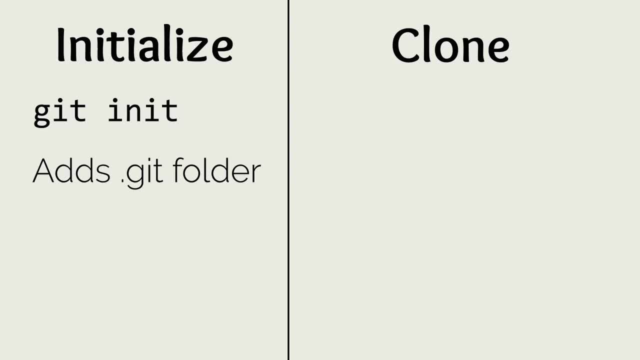 url and not the http url. Now, with that url copied, type the command git clone into the terminal with the copied url at the end of the command. This will copy all the code from the repository onto your computer and set up Git to track the changes. This also adds the remote repository. 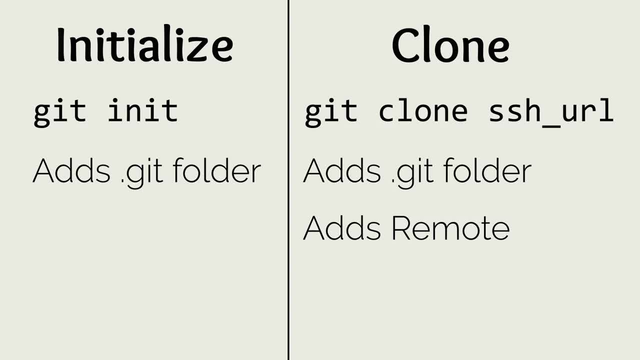 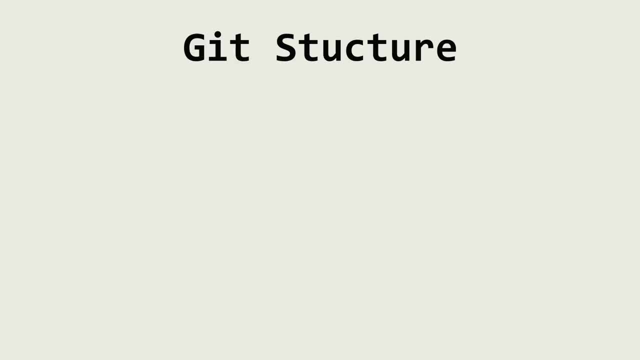 to your Git config for the project so that when you are ready to push your changes to GitHub, Git will already know where to push them to. Now that we have a project set up on our computer, let's talk about the structure of Git. 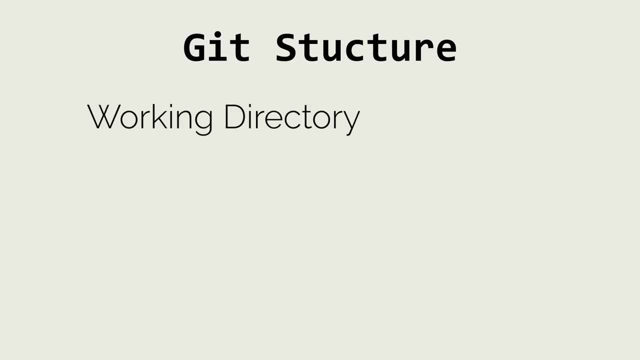 Git tracks changes through three stages: the working directory, index and head. The first stage is the working directory. The working directory is simply all of the files in the local repository in their current state. None of the changes in the working directory are tracked. 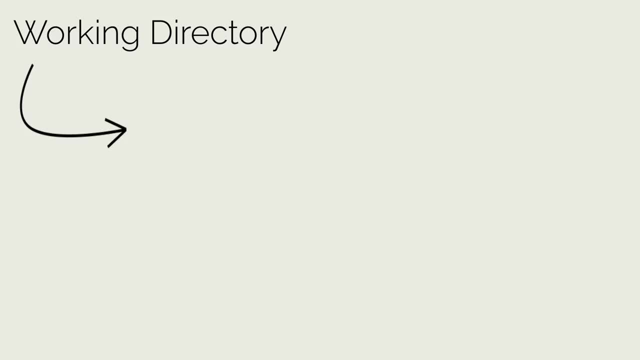 by Git. In order to track these changes, we first need to add them to the index, which is commonly referred to as staging. This can be done by using the git add command. This process of adding changes to staging tells Git that we want to track all of the changes that we have made in our working directory. 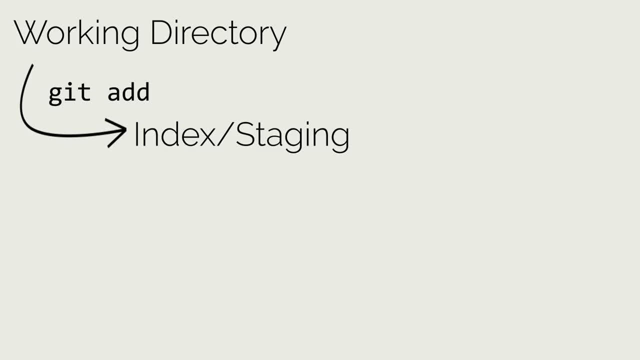 This still does not make these changes an official version of your code that you can change between them. In order to add these changes as an official version, we need to tell Git to commit these changes from the index to the final stage, the head. This tells Git the changes are final and. 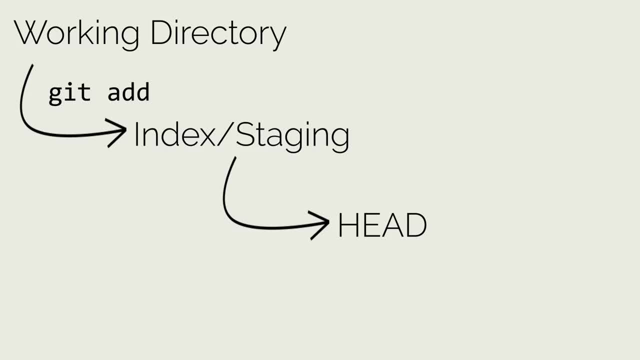 requires a message to be saved with the commit. This can be done by using the git commit command. The head is simply the most recently committed version of your code. After committing changes to the head, they are saved as a version on our computer. 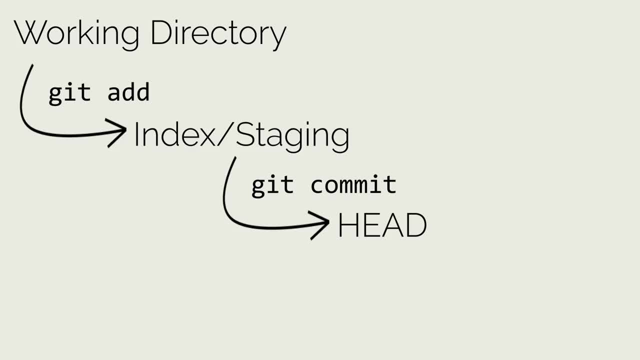 but they are not in our repository on GitHub. In order to get these changes to our remote repository on GitHub, we need to push them to GitHub using the git push command. If you set up your project using git clone, then Git will already know where to push these files to. 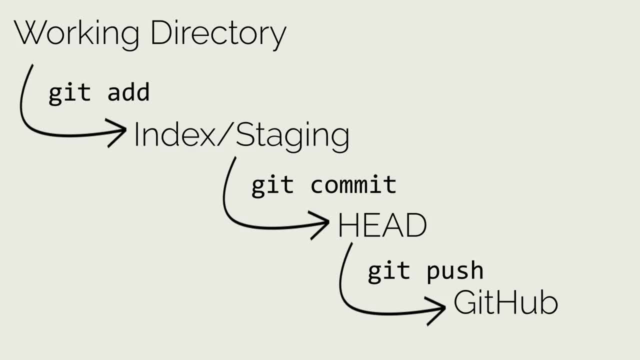 But if you used gitanit to start initialize the new project, then tagging will need to be told where to push. the changes to. This command is basically the code that will be delivered to your Silverplate repository and what it means to be active on your之後 brain For the Github repository. 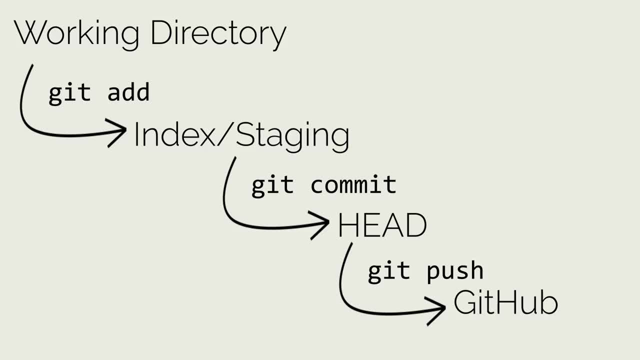 you can also be able to allow Git to warm up your files and add changes to themwiek if it's called information on the command. This can be done by creating a repository on GitHub and copying the SSH URL for cloning. After that is done, you can simply use the git remote add origin command with the copied URL at the end of the command. 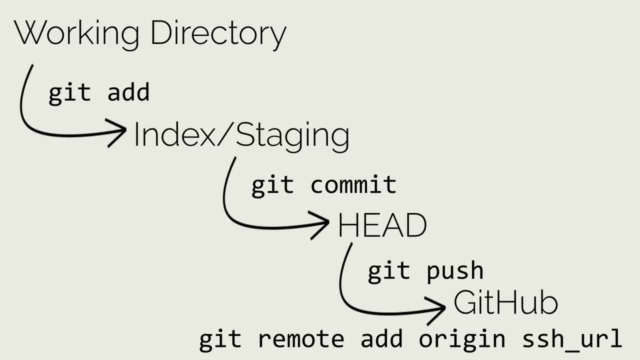 This tells Git that we have a remote repository called origin at the copied URL. With the remote repository added, you can use the git push command to push the changes to the remote repository on GitHub. We now are able to create a repository, make changes to it, save them and push those changes to GitHub. 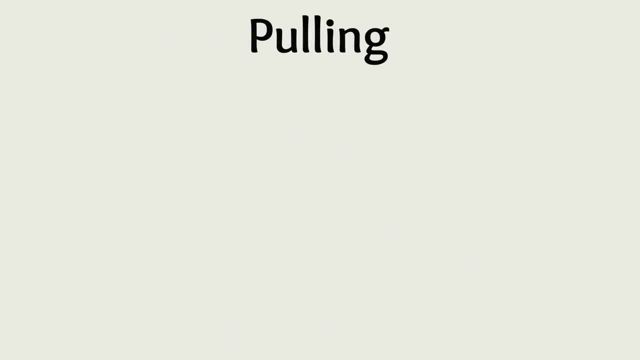 But what if another one of our team members wants to pull down the changes that we push to GitHub onto their local computer? This is where the git pull command comes in. By simply typing the command git pull into their terminal, all of your changes from GitHub will be pulled onto their local computer and merged with any of the changes that they have. 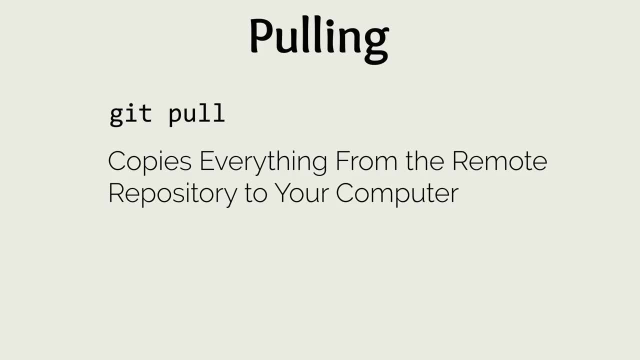 That is all you need to know about Git in order to get started. but there is one more big concept in Git. It is called branches. Branches are essentially a copy of the code at a point in time that has its own, separate history from the main branch, which is called master. 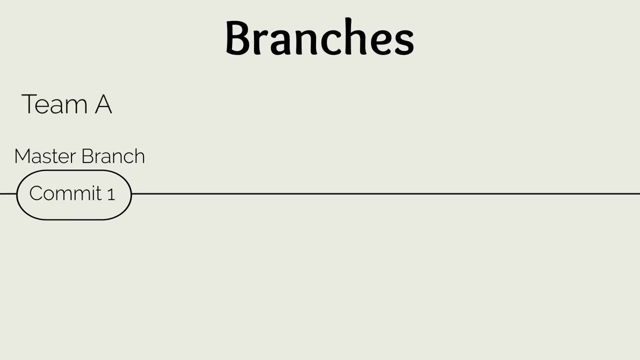 Imagine you are in a company with two teams and one of the teams is creating feature A of a website and the other team is creating feature B for the same website. These features will have multiple commits in order to be fully completed, but if both teams are working out of the master branch, 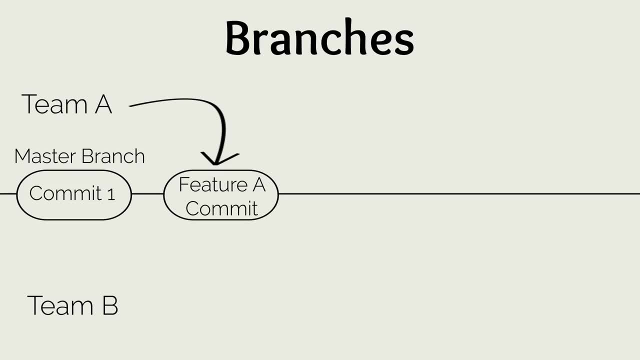 then whenever the team working on feature A pushes their changes to GitHub, the other team will get those changes for feature A when they try to pull. This will cause problems because now the team working on feature B will have parts of feature A in their code. 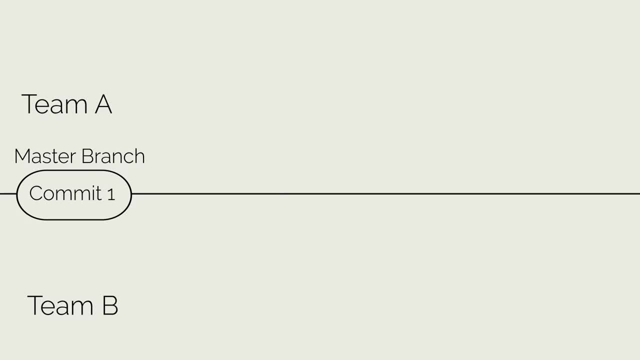 This is where branches come in. If the team working on feature A creates their own branch off of master and the team working on feature B creates their own branch off of master, then when the teams push their changes to GitHub, they will only be pushing their changes to their own branch and not the master branch. 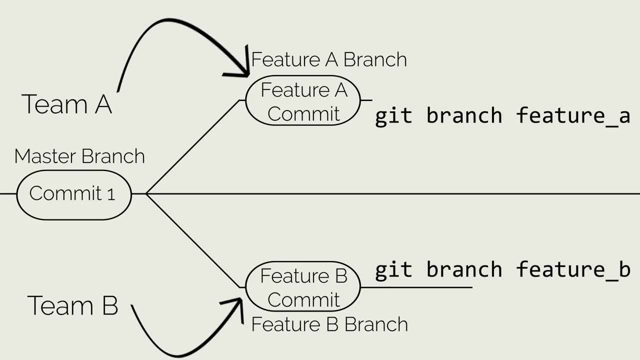 This can be done using the command git branch, with the name of the branch being created at the end of the command. This will create a new branch, but in order to switch to that branch, the git checkout command will need to be used with the name of the branch at the end of the command. 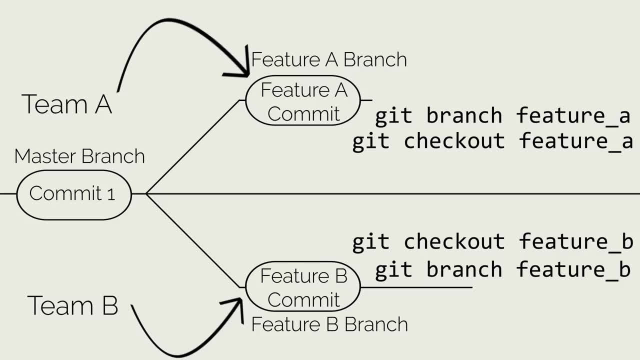 Since this is such a common operation, there is a parameter you can pass to the checkout command to create a new branch and swap to it. This command is git checkout dash b with the new branch name after the dash b. Now that both teams have created their own branches and committed all of their changes for each feature to their branches, 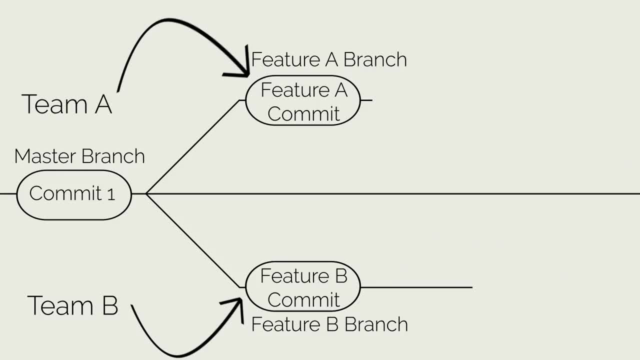 it is time for them to merge these changes back into master. Git makes this easy with the command git checkout. Git merge, followed by the branch name that you want to merge will merge all of the changes from that branch into the branch you currently have checked out. 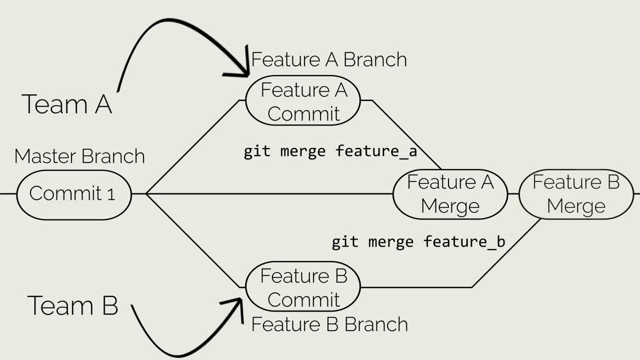 If there are any conflicts between the two branches, git will notify you of these conflicts and let you decide what to do with them before committing the changes. This is, finally, the end of all you need to know about git. I know it can seem quite daunting, but I am going to go over a live example of exactly how all of these commands work to give you a more hands-on experience with how git works. 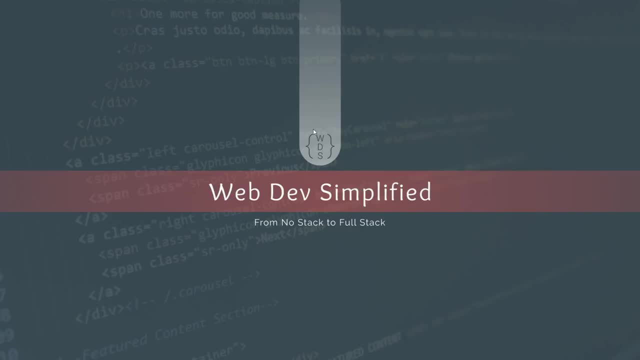 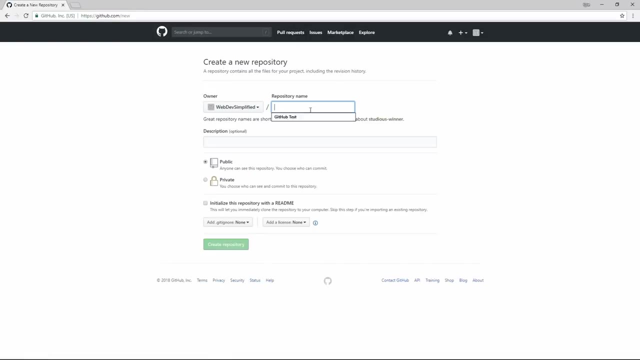 Let's jump into that. Hello everyone, Let's first get started by setting up a project on git. The easiest way to do this is to go to github, create a new repository. give it any name you want. We're just going to call ours github-test. 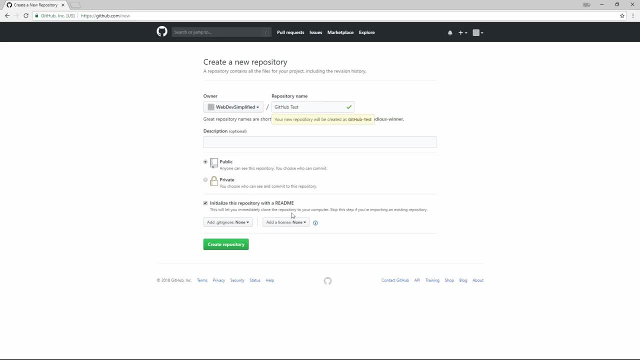 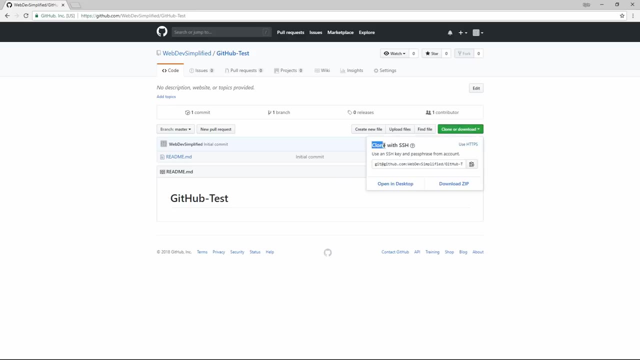 And then click to initialize this with a readme. This will make it so that you can clone the project down to your computer And then click create repository And after that's done, loading it will bring you to your repository page. Here is where you can clone the URL and make sure you use the ssh URL. 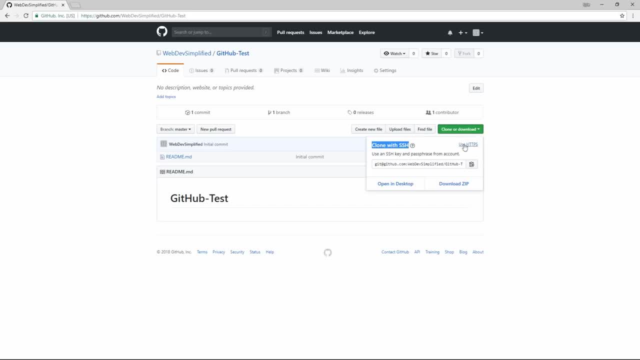 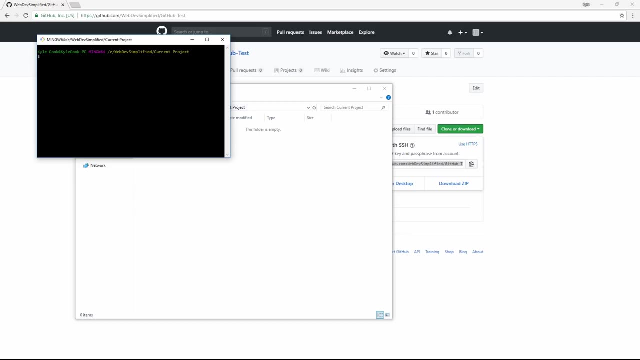 If this says clone with http, make sure you click the button up here which will say use ssh. After you're done with that, click the URL, copy it and then go to the folder that you want to copy this into. Once you're here, you can right click this and open the terminal here. 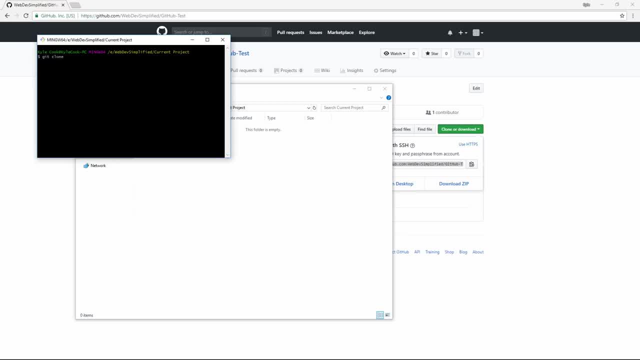 And then all you need to do is type git clone and then paste in the URL that you just copied: Hit enter for this. We'll copy all of the code that is inside of that repository, which includes that readme we created, And bring it into the folder that you are in currently with the terminal. 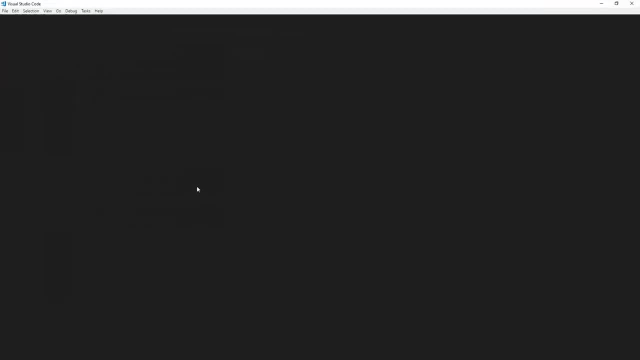 Now to open this, just right click it and open it with Visual Studio Code And we can get started right away. and we see we have a readme And it just says the project name. The readme is important in version control systems such as github. 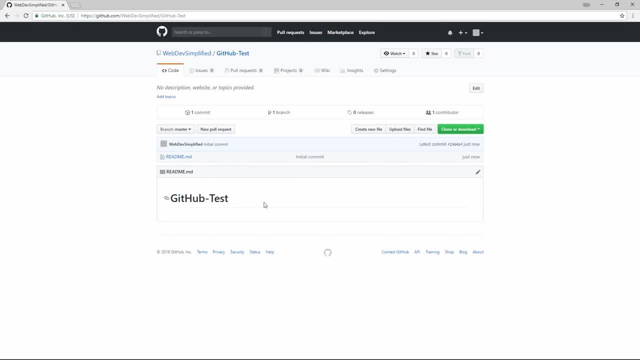 Because if you go to github's site, you can see that inside of your repository, everything in the readme will show up on the main page of your repository. This is a great place to put notes and information about what your code does, So that when people come to your repository they have an easy way to understand it without having to read the actual code. 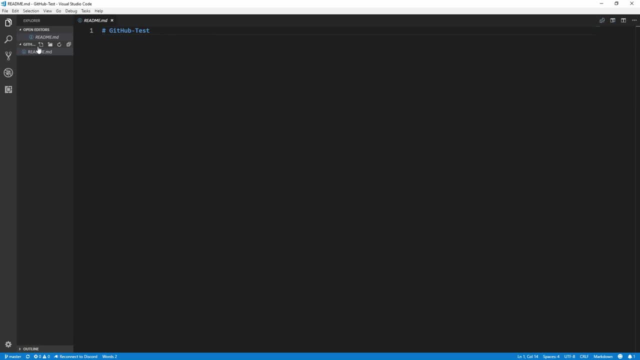 Now that we have that out of the way, let's get started by creating a file in this project. We can call it anything we want, such as testhtml, And hit enter. After a little bit you'll see that this file will turn green with a little u next to it. that stands for untracked. 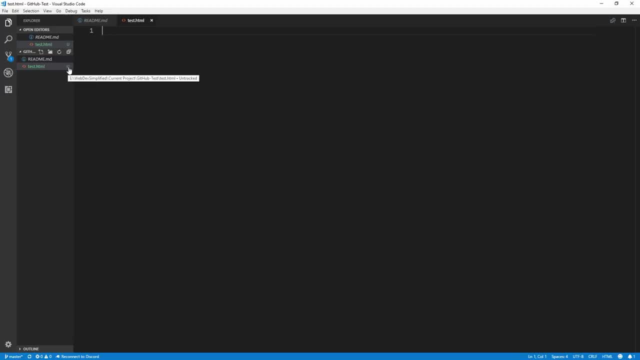 This is because Visual Studio Code integrates perfectly with git And this tells us that this file, which is green, Means that it is new And since it has a u saying it's untracked, that means we haven't added this file to our git repository yet. 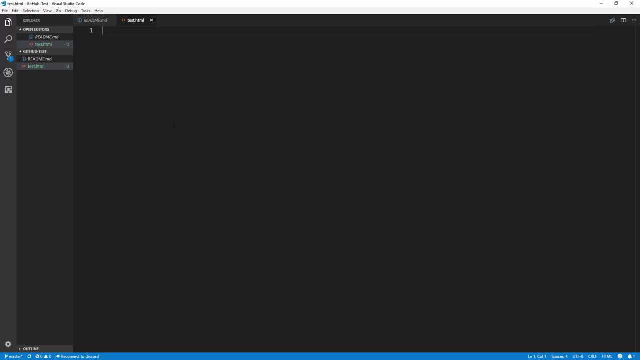 In order to do that, let's open up the terminal by holding control and hitting the tilde key And typing in git add. What we'll need to do is add the file name to the end of the git add command to tell git what we want to add. 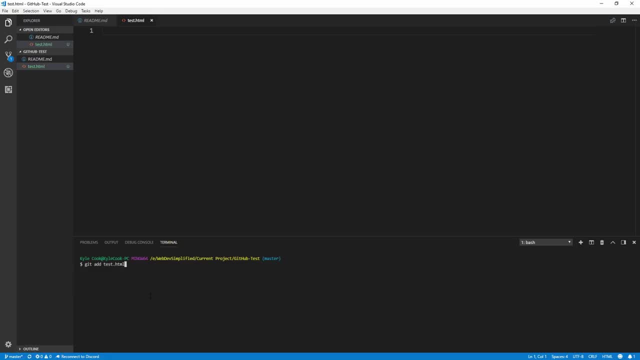 So we'll say testhtml. This will add the testhtml file to the index of our git repository. When we hit enter, We'll see that this turns to a instead of u, which means it's been added to the index. And then, lastly, if we want to commit this change, we can type git commit. 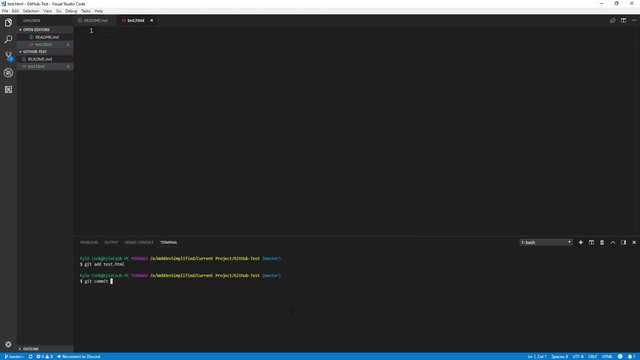 And then we need to add a message to this. So use dash m to say that we're adding a message And then in quotes put whatever message you want, such as added test file, And then hit enter And this will add this file to our repository. 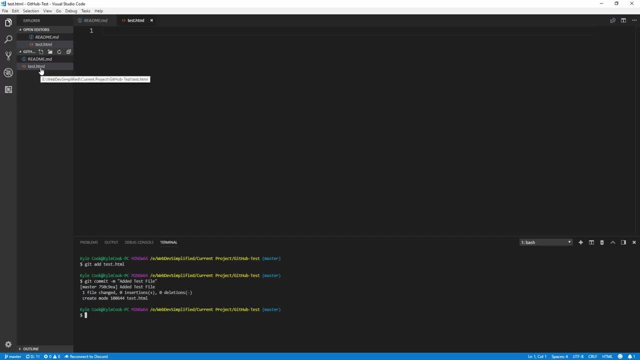 And you'll see that it is no longer green anymore Because it is being tracked by githtml And it is in an actual commit. Now let's say that we want to edit this test file By adding some constant in here. Let's just say we're going to add a paragraph tag. 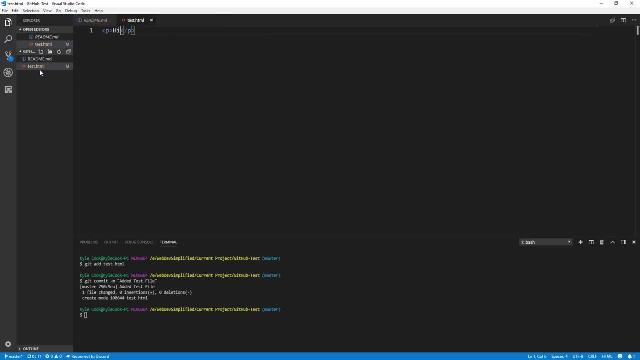 And we're going to put high inside of it. If we save that, we'll see that this will turn yellow Or orange, Which means that the file has been modified. as you can see by the m, This means that it is different than the current version in git right now. 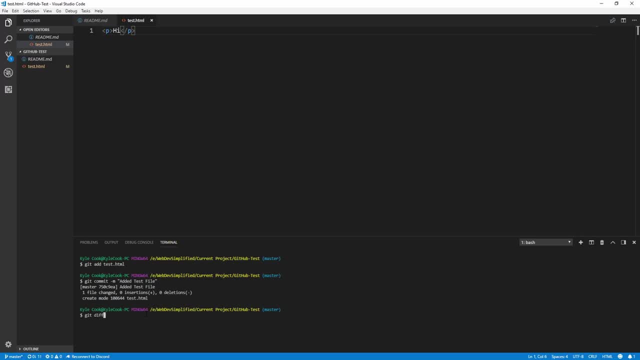 In order to see what's different between these two files, we can run the git diff command. This command will tell us everything that is different In the files that we have in our repository Between the current version that we have in our working directory. 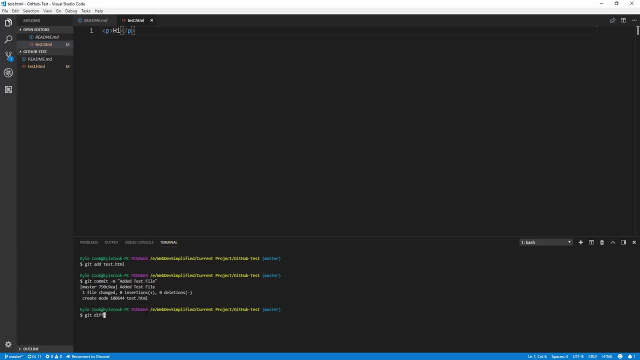 And what is the most recent version in the head. So if we hit enter, we'll see that it tells us that this file The testhtml. The only difference is that we added this line high, Which is what the green stands for. 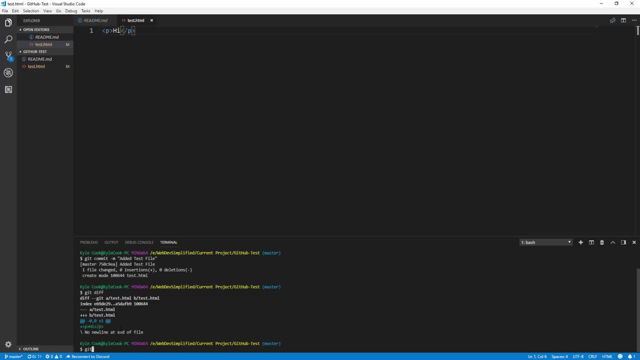 It means that it has been added. Now let's add that to our repository And, instead of using the file name, we're going to use a period Which tells git that we want to add it. We're going to add every single file that is in our project. 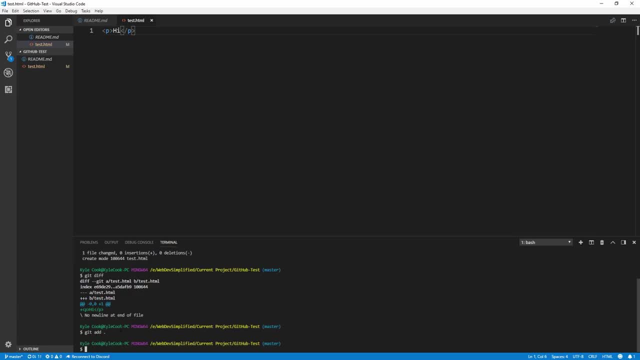 This is an easy way to add a bunch of files at one time. So when we do that, we'll see that our file will get added here, And then if we want to commit that, we do git commit. Give it a message. 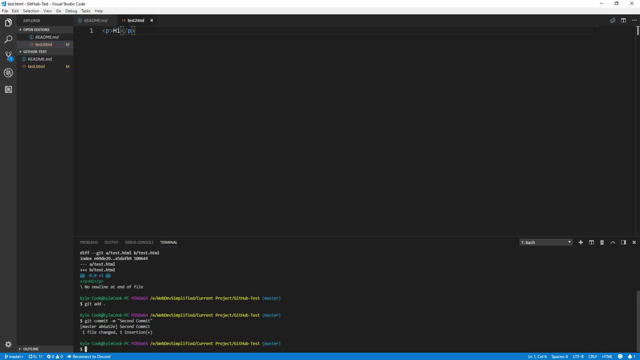 We'll just say second commit, Hit enter And now our file will be added. With git we can make as many changes to as many files as we want in the project, And as soon as we add them they will all be added into the index. 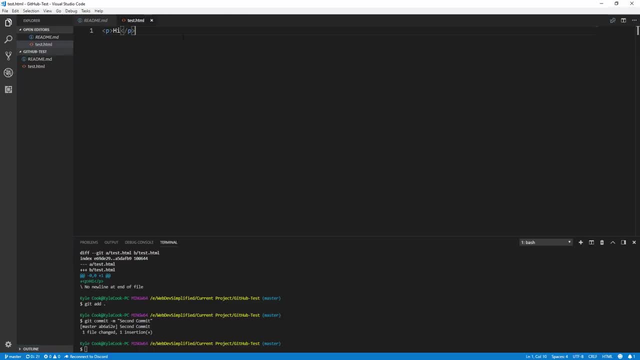 We can even add multiple different times. For example, we want to add another p tag here And just say content, And then we want to add that. So we do git add and put the period at the end, Hit enter, And now let's say we're going to change it again before we commit. 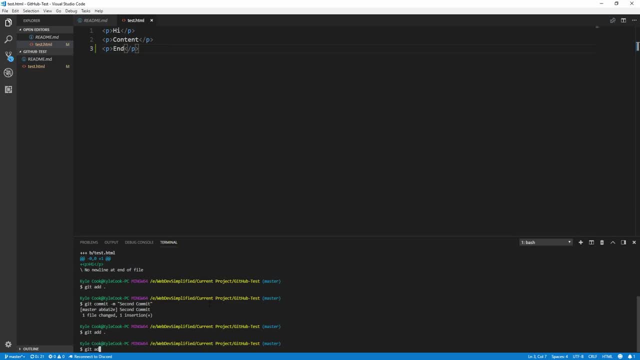 And we want to put an end here. So we can do git add with a period at the end, And now that's added to the index as well. So you can do as many adds as you want in between commits And now when we say, okay, we have all of our changes that we want. 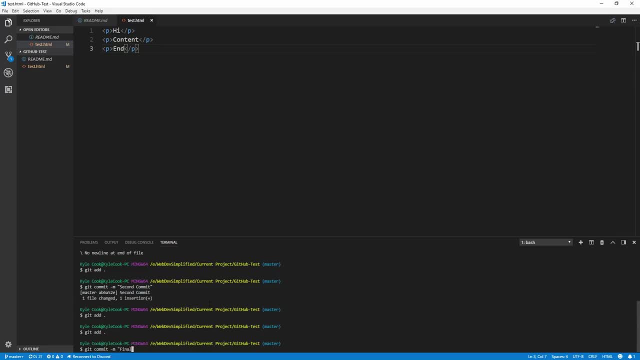 We can say git commit, Send it a message of final commit And we hit enter. We'll see that this file will no longer be marked as modified, because it is actually in the head of our project. Now that that's out of the way, let's push our changes to GitHub using the git push command. 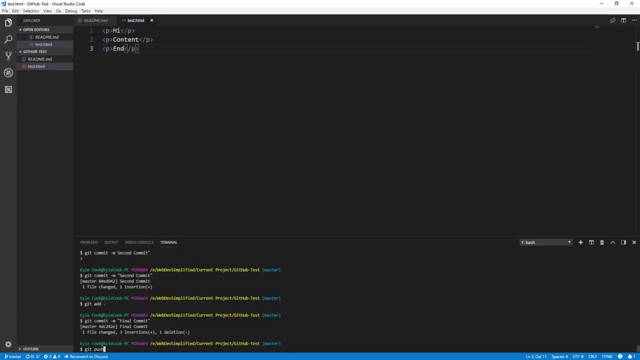 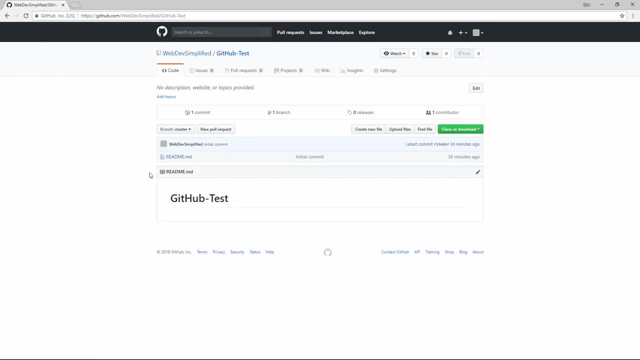 If we have git and GitHub configured correctly, this command will automatically push all of our changes to our remote repository. Let's first look at our remote repository, refresh it and see that none of our changes are currently here. In order to get our changes to show up there, we just need to run the git push command. 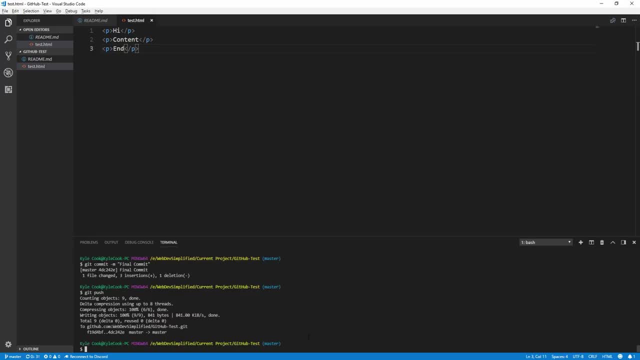 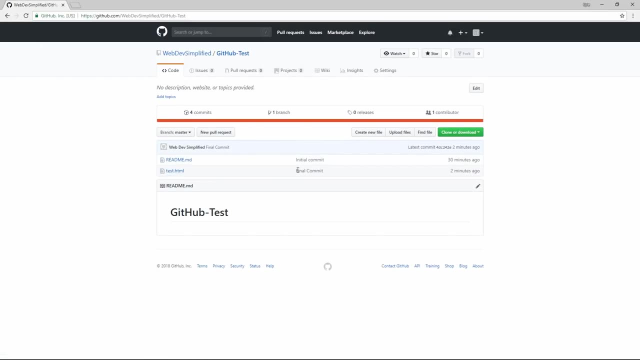 If we hit enter now, this will push all of our changes to our remote repository And if we head over to it, hit refresh, we'll see that these changes are now here And it shows us the commit message that we sent with it as well. 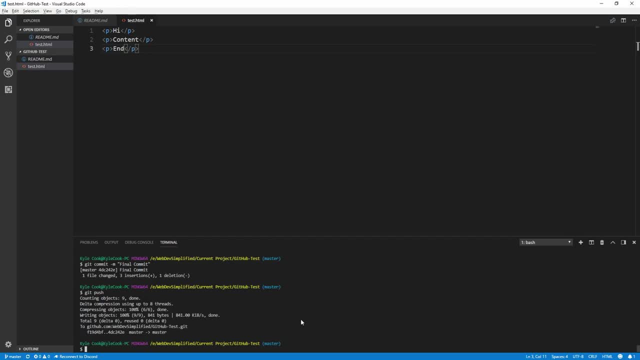 Now let's go back to here and get started on git branches. The first thing we need to do is to create a separate branch for a new feature that we're going to create. So let's say that we are going to create a feature that allows us to take payments. 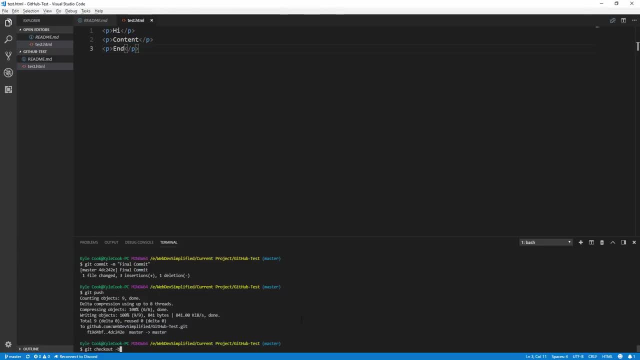 So we're going to want to create a store, So we'll use git checkout, dash b and the name of our branch, which we will just call store. Now we have transferred over to a separate branch, As you can see in the bottom left hand corner. here, Visual Studio Code tells us exactly what branch we are on. 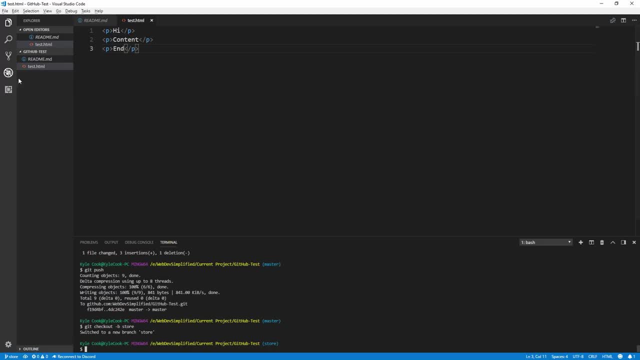 It says store right here, so we know that we're on the store branch. Now let's add a file in here called storehtml And let's add some content. We'll just add a paragraph tag in here that says this is the store. 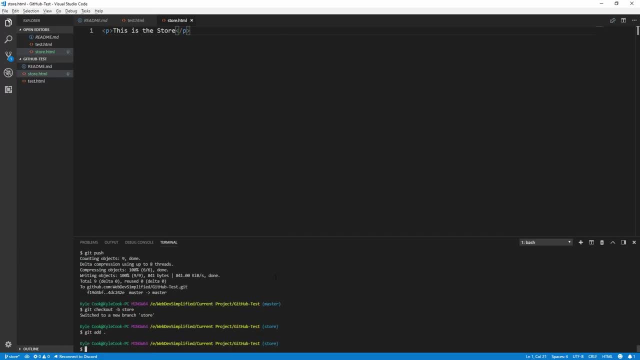 Now we're going to save that And then commit that by saying added store. And now we want to push these changes. so let's do git push And we'll see that it says there is no branch currently on GitHub for this project, because we don't actually have a store branch already on GitHub. 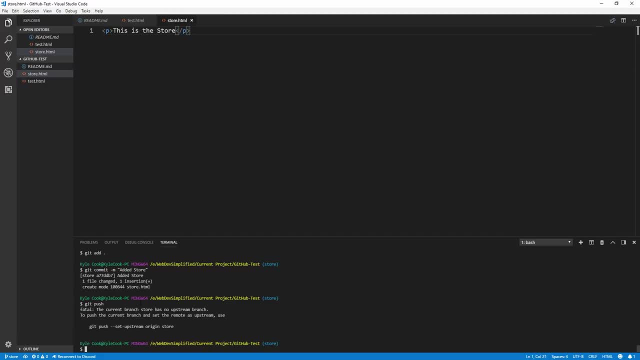 What we need to do is we need to tell GitHub to create this store branch. In order to do that, all we need to do is copy this command, which will configure git in GitHub so that it is able to pull and push to the correct branch. 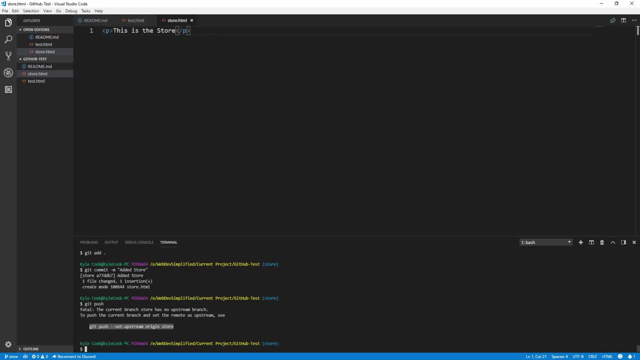 So now that git and GitHub both know that this branch exists, Let's paste that in here and hit enter, And we'll see that it will push our changes up to our remote repository. Now let's go over to our remote repository, refresh it and you'll see that these changes don't actually show up. 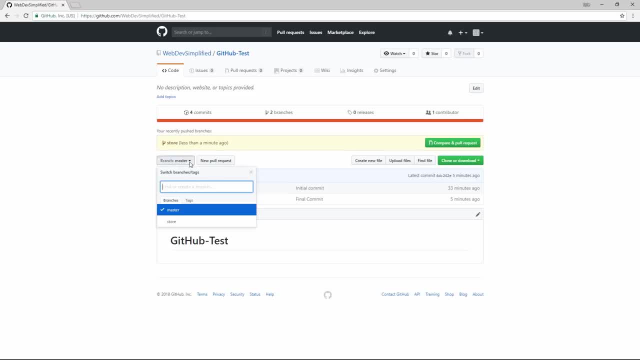 It's because it's on a separate branch. As you can see, here we are on branch master And if we switch to the store branch, you'll see that now our store changes show up here. If we switch back to master, you'll see that they are no longer there. 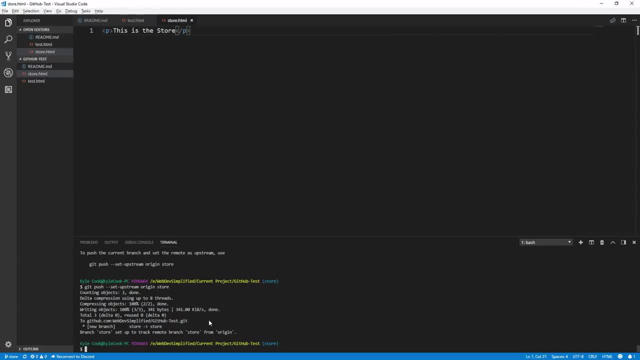 But we want those changes to be in master, Because now our store is complete. In order to do that, we need to switch back to the master branch by calling git checkout master, which now switches us back to the master branch, And we can see that down in the bottom left here in Visual Studio Code. 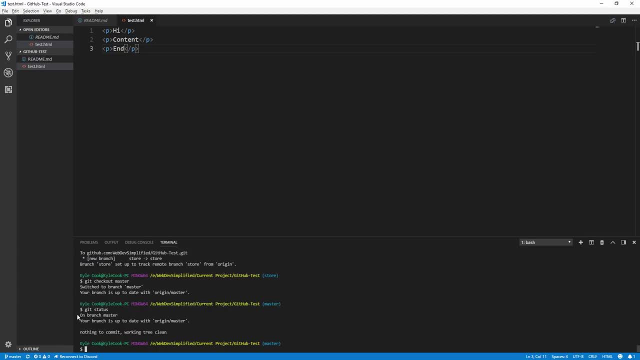 Or if you just hit git status, hit enter, it will tell you exactly what branch you are on. So now we need to run the merge command to merge our changes from our store branch into our master branch. So we type in git merge. 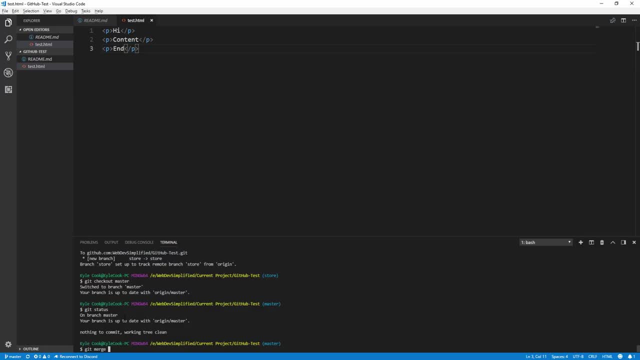 which will tell git to merge whatever branch we mention into the branch that we are on, which is the master branch. So if we type git merge and the name of the branch which is store, hit enter, all the changes from the store branch will be merged into our master branch. 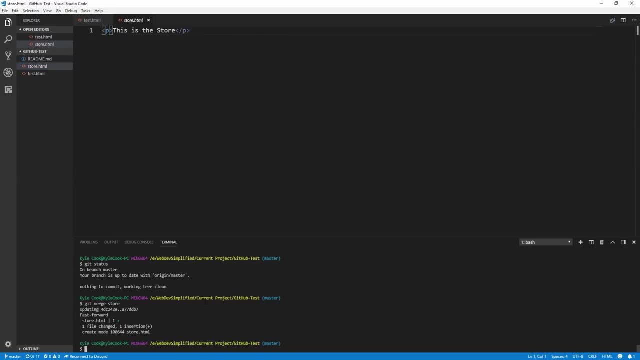 And, as you can see, the storehtml pages showed up. So now, if we run git push in order to update our remote repository with our local changes and hit enter, you'll see that now when we go to our remote repository and refresh it. 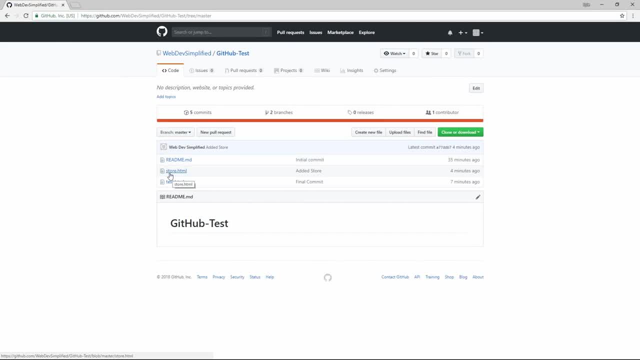 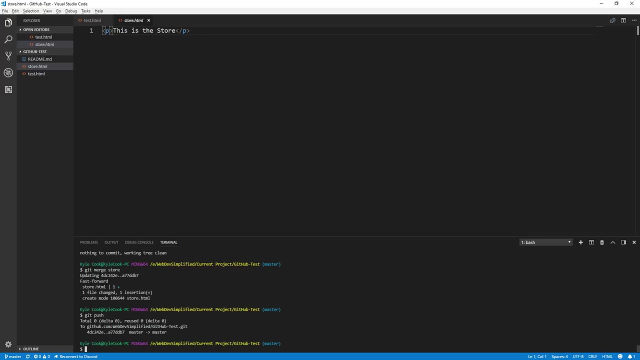 that the store page is now there. This is because the merge command automatically adds and commits the files with a message that says that it has added the store. Now, if we go back, what happens? if there is a merge conflict, though? Let's say we have, this is the store and in our master branch we change this to say this is the store 2.. 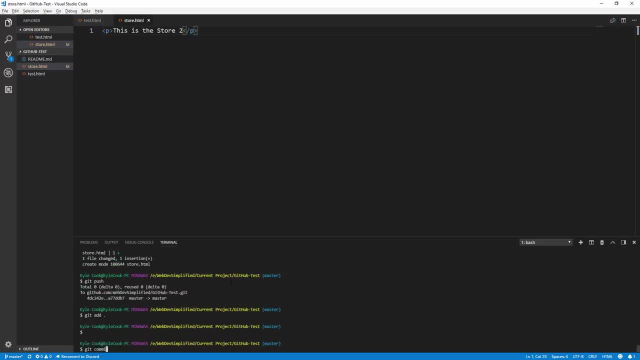 And if we add that and if we commit that with just any message and now we switch back to our store branch, which we can do with git checkout store, Now we are back on the store branch and, as you can see, this is updated to be: this is the store. 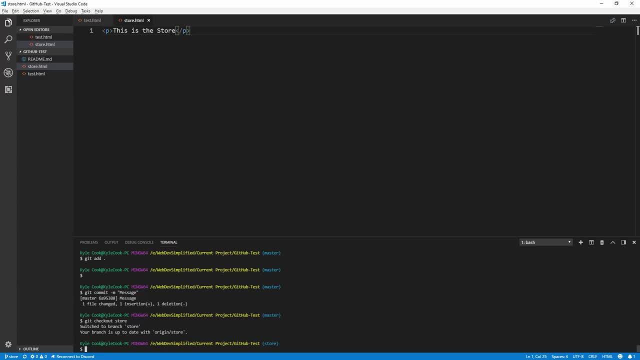 since we do not actually have those changes for master on this branch And let's say we change this to be: this is the store 1. Save it, add those changes and commit them. Any message will work. And now let's switch back to the master branch. 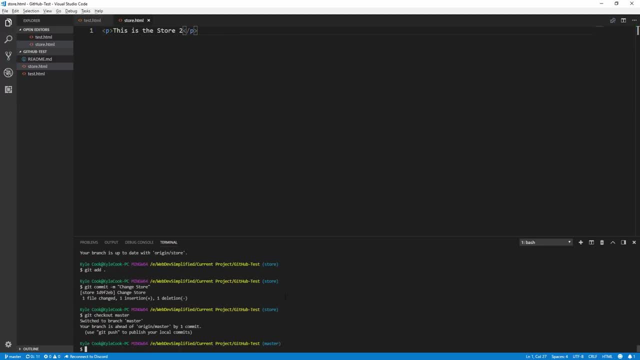 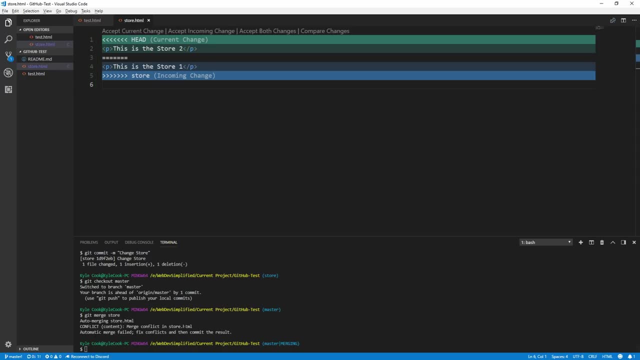 So now what we want to do is we want to merge those changes from our store branch into our master branch, just like before, by calling git merge store. But you'll see, right here it tells us that there is a conflict and it is saying that inside of the storehtml file there is a merge conflict. 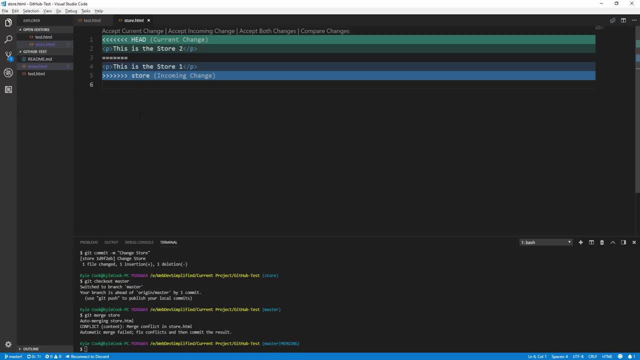 And Visual Studio Code will very nicely highlight this for you, but git also will add in these less than signs followed by head, as well as the greater than signs followed by store, telling us that the head is our current branch. so everything between these equal signs. 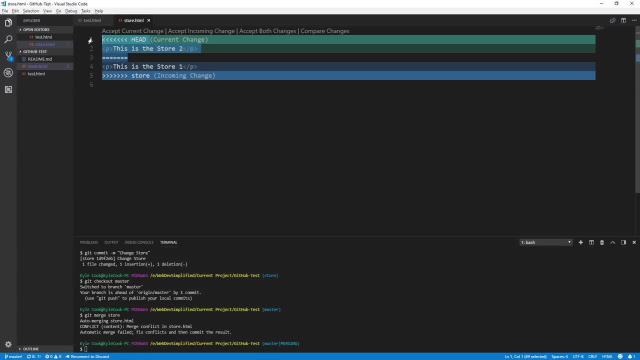 and these less than signs is what is on our current branch, and everything between the greater than signs and the equal than signs which is from the store branch will show up here And it's telling us that git is not smart enough to know which change it wants to add in. 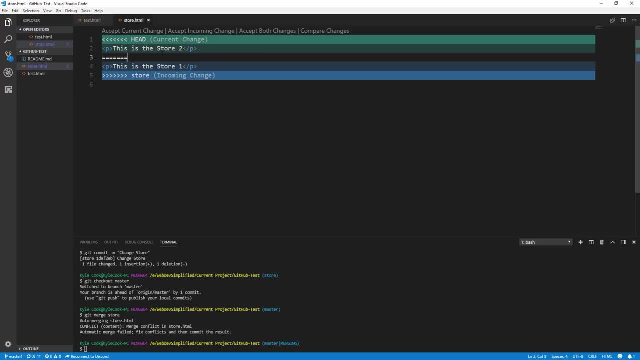 It is saying that we need to figure out which change should be saved. So all you need to do in order to decide on what change is going to be made is you look at it and say, oh okay, well, we want this as the store. 2,. 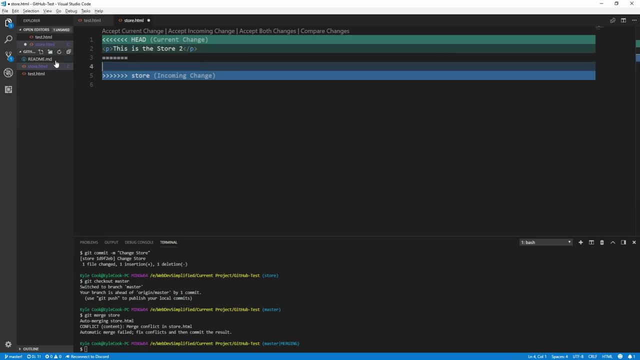 we don't want this as the store 1, so we delete this as the store 1, as well as all of the signs that git creates. So if we delete that, delete these. make sure we got it all set up with no extra line breaks in there. 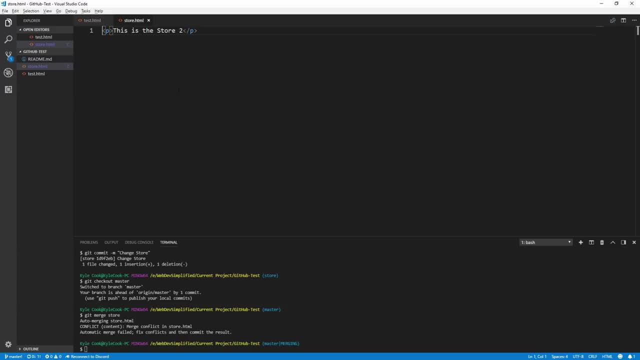 save it, and now we have decided on what conflict we want to add in. So what we are going to resolve from, we've decided that we want to take the changes from the master branch and none of the changes from the store branch. 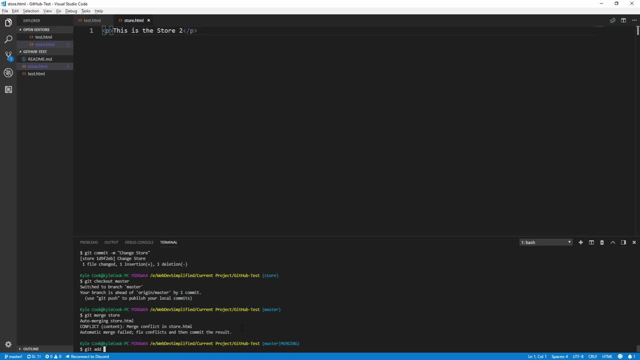 Now all we need to do is add that file by calling git add, with a period after it, and then we can just call git commit. This is because git will automatically generate a commit message for us if we hit enter, As you can see. 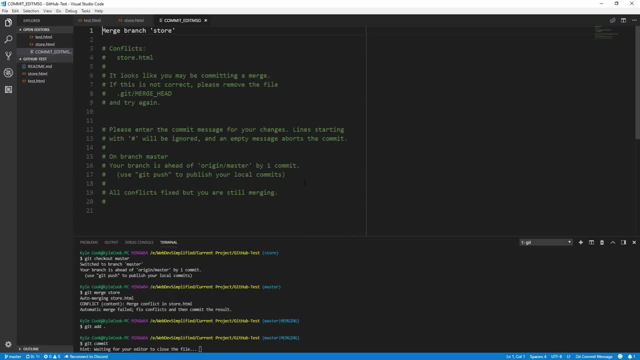 it opens it up in Visual Studio Code Editor, which is something that, if you watched my video on setting up git in GitHub, was an option that I gave you, as opposed to using the terminal. Once you have gotten in here, we see that git has already created a message for us. 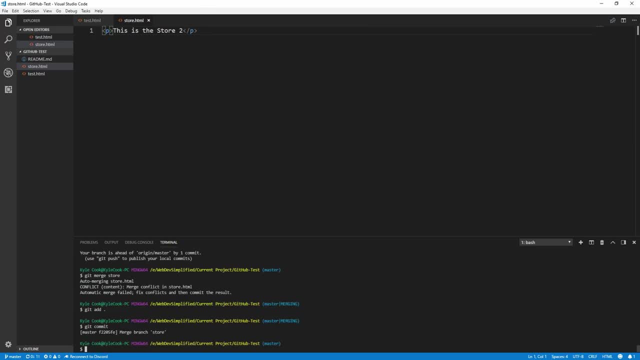 so all we need to do is save this file and close it, and it will automatically create that merge for us. Now, if we git push, set it up to our remote repository, you'll now see that when we go to our remote repository. 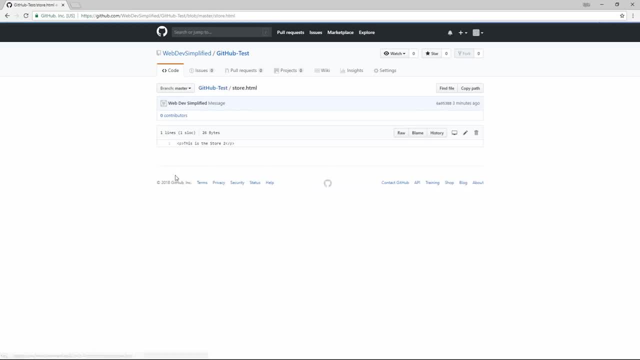 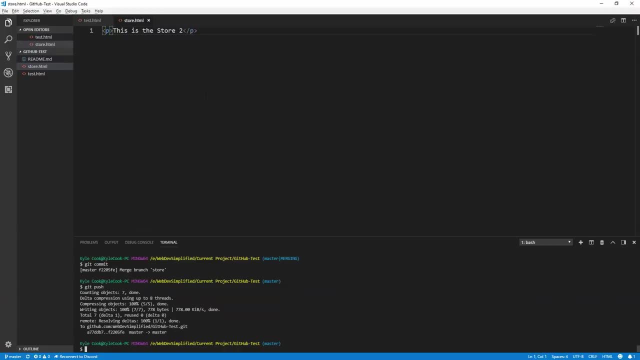 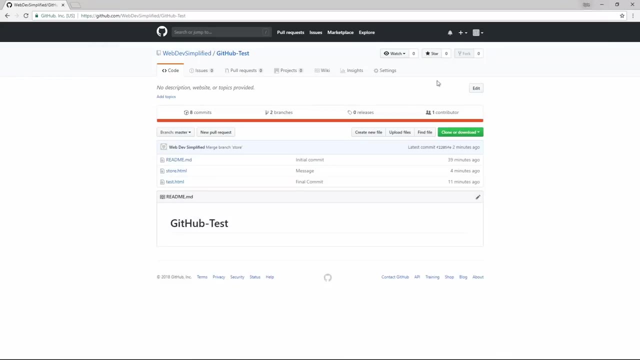 refresh it and we open up our storehtml page. we have. this is store 2,, which is exactly what we wanted in here. Now, in order to simulate having multiple people working on the same project, I'm going to reclone this project. 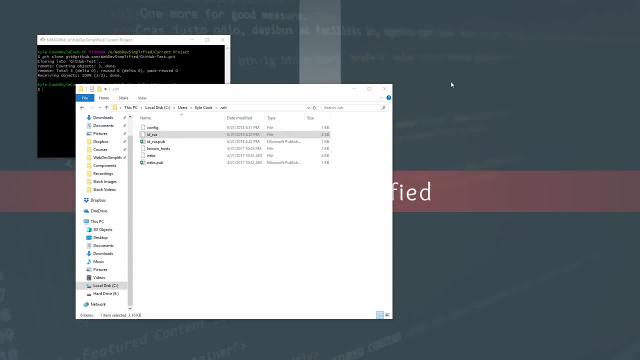 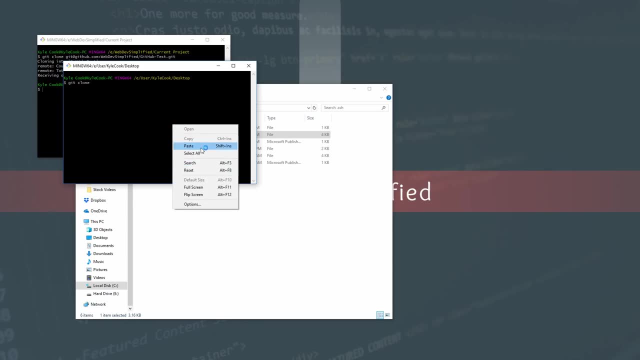 copy the URL here and I'm just going to clone it onto my desktop. So if I type in the git clone command, followed by that URL, hit enter and now it will clone that onto my desktop and you'll see that if we open this up. 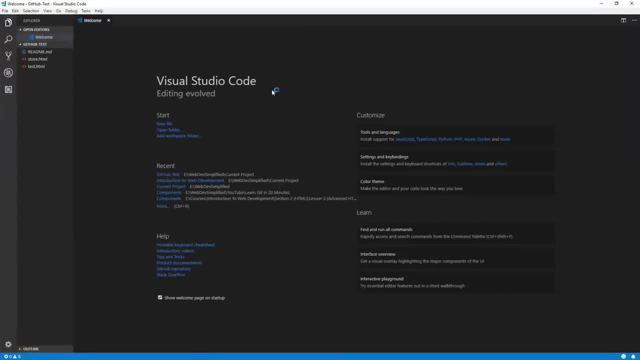 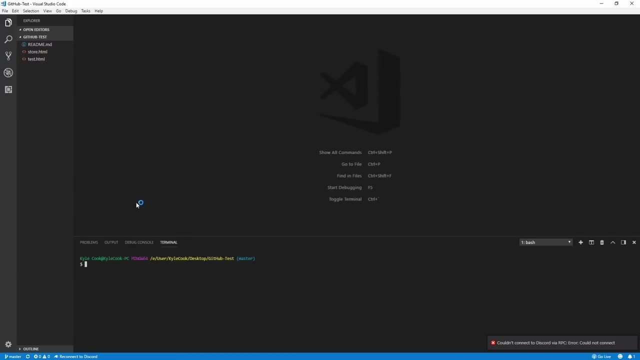 using Visual Studio Code. we have all of the changes from before. So now let's open up the terminal and imagine that we are now a different developer working on this project, And let's say we come in here and we want to add another line in here that says: 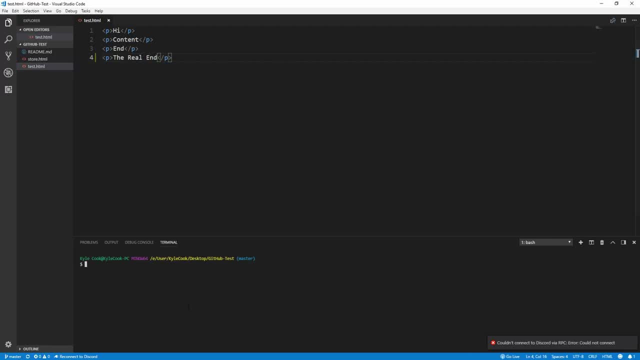 the real end. Save that. let's add that with a message that says John's Changes, because we're going to be pretending that we are John, and let's push that up to the repository. And there we go. Now, if we go over to our repository, 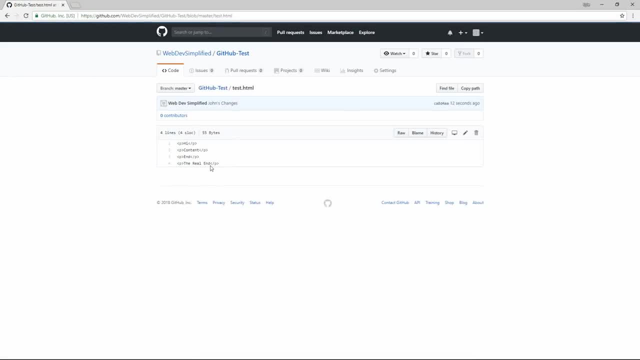 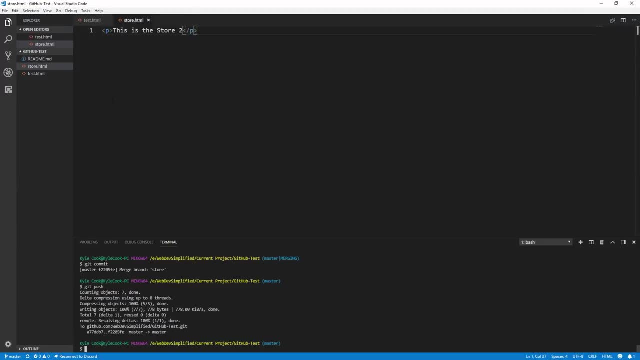 refresh it, you'll see that this test has John's Changes at the end here. But if we go to our original project, this one that is open inside of, not the desktop, this is the original one that we created. you'll see that when we go to the test. 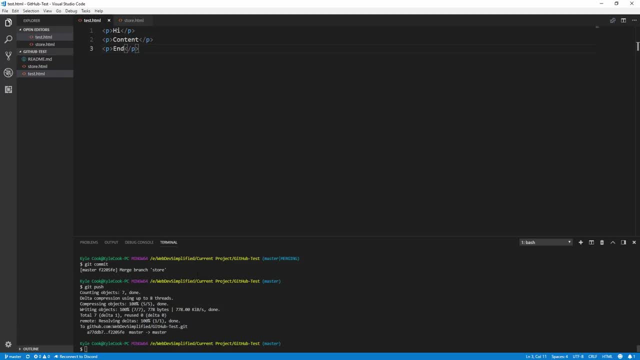 John's Changes are not here. This is because we need to use the git pull command to update our local repository from the remote repository. All we do type in git pull, hit enter and it will pull down all of the changes from the remote repository. 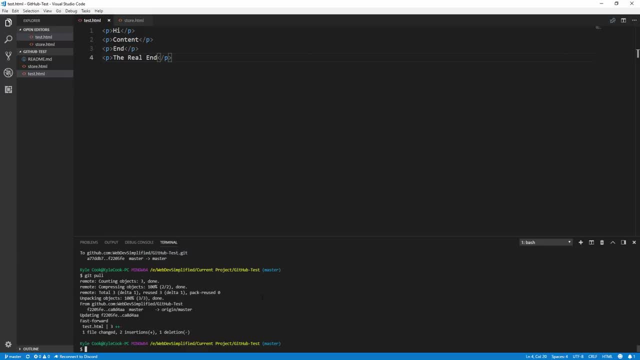 for the branch that you are on And since we are on the master branch, it pulled down the changes from the master branch, which is where John added his changes. That about sums up everything that you need to know about git. The whole process goes. 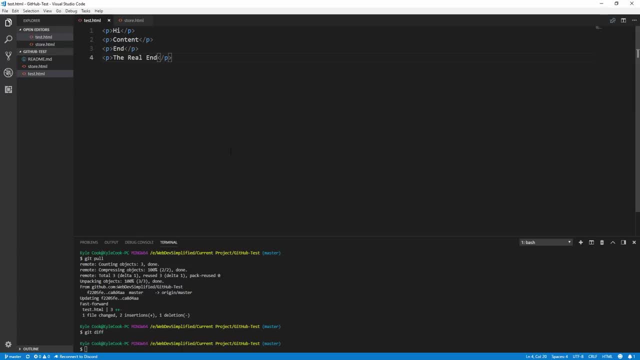 first create a project on GitHub. next clone that project down to your local computer, add any amount of code and changes that you want using the git add command and once you finalize those changes into a coherent version, use the commit command to commit those changes to git. 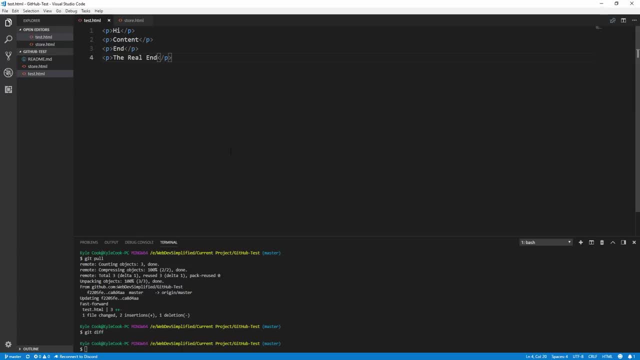 And then, lastly, after you've done all of the adding and all of the committing that you need to do for a particular feature or project, then you use the git push command to push those changes back up to GitHub. You'll also need to use branches in between there. 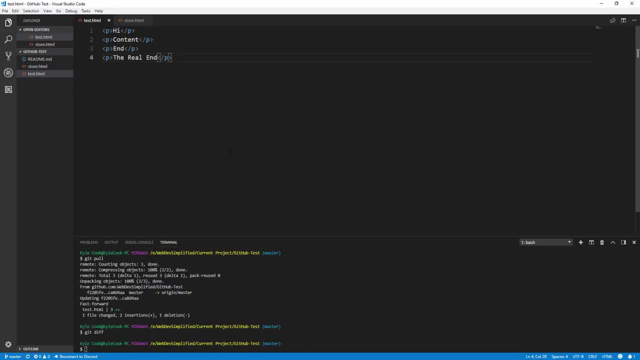 to be able to create new branches for certain features, so that you do not bring different features into each other. instead of using just one branch- the master branch, for example, where all of the features would be- you now have separate branches for each of your features. 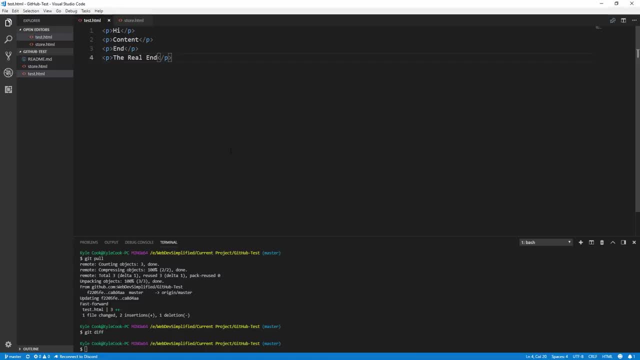 so that your code does not get mixed together and then at the end merge those back into master, since master is your overall branch. that describes the current state of where your project is, And that's all there is to it, If you liked the video. 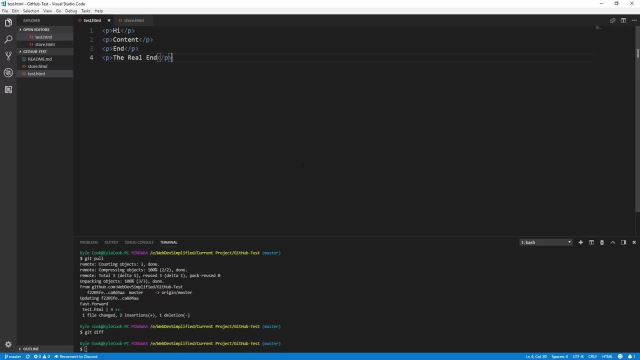 please remember to leave it a like and subscribe for more content, and if you want to see a more in-depth tutorial involving some of the features of git that I was not able to cover in this video, please make sure to comment down below letting me know.